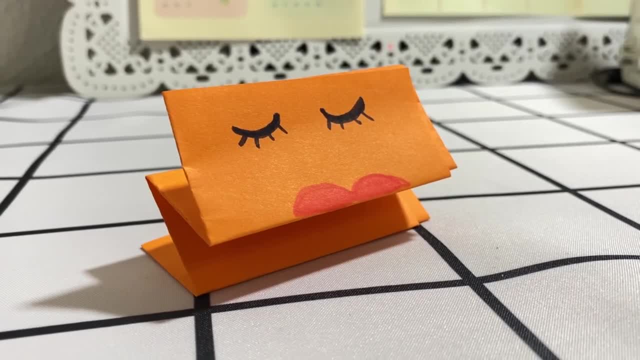 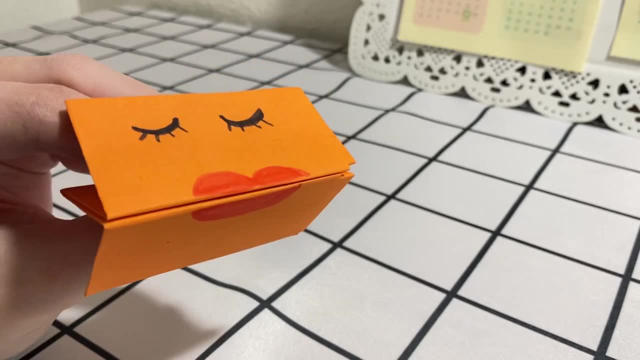 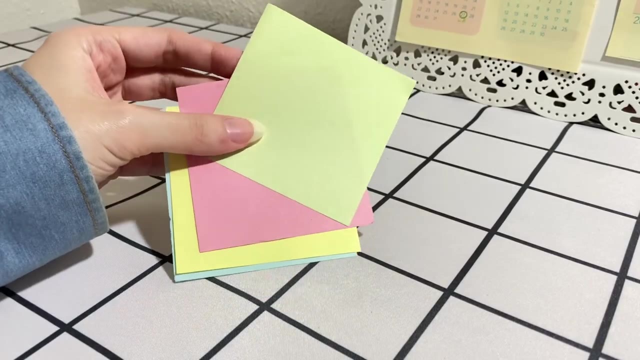 These puppets can be used for telling stories or answering questions, Pairs can practice together a conversation or groups can make a puppet show. Our second craft is the 3D house. For this one, each student needs four pieces of paper. I'm using these tiny papers just for the puppet. 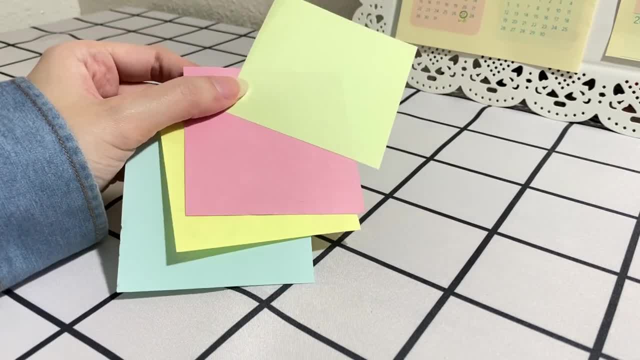 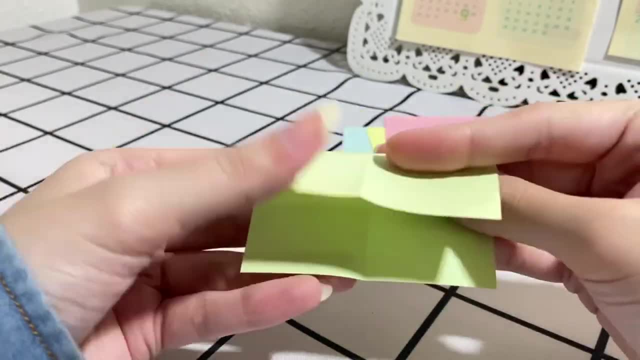 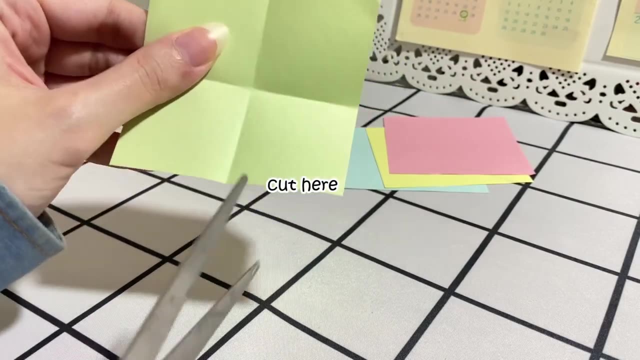 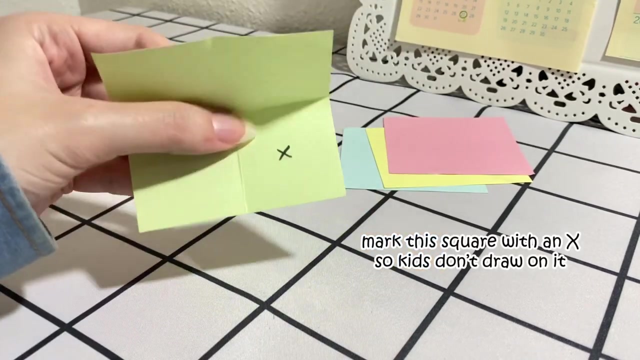 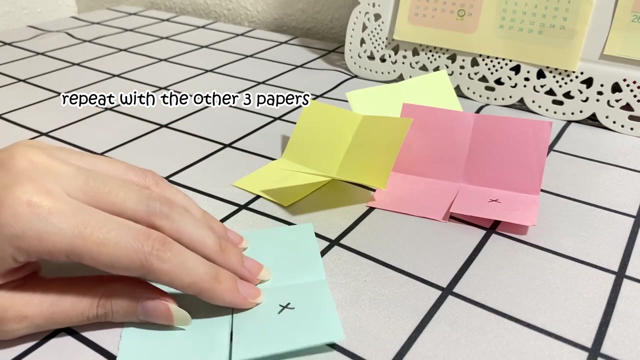 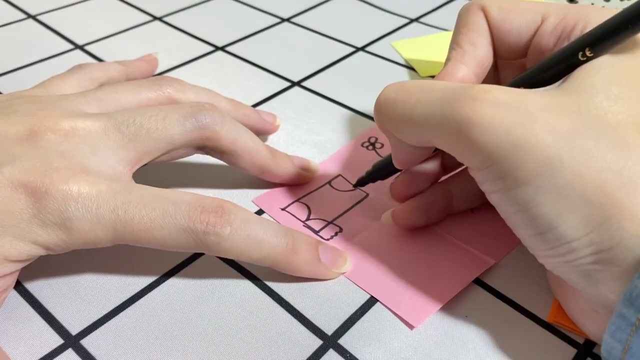 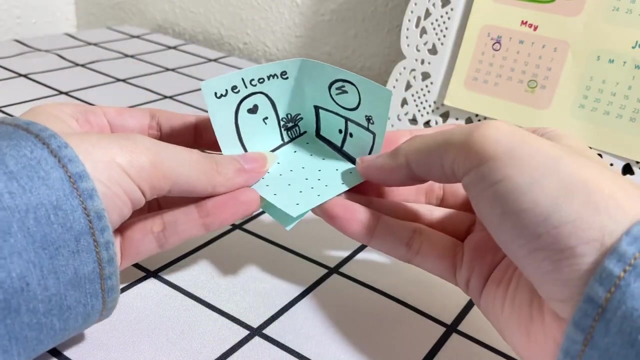 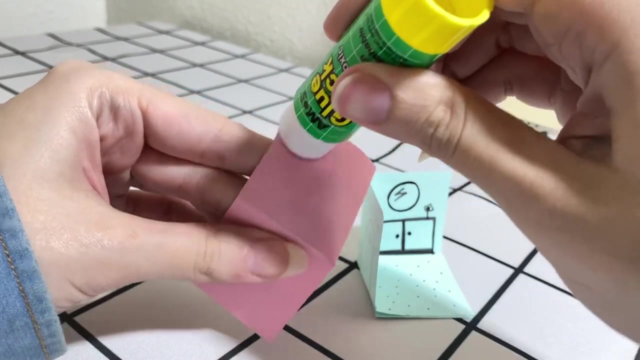 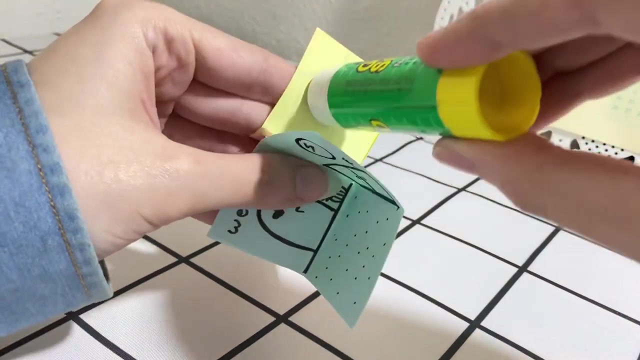 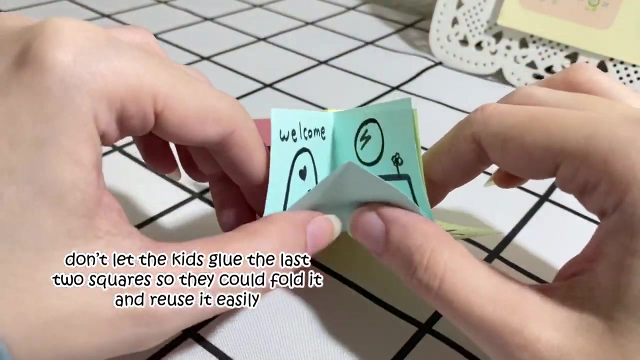 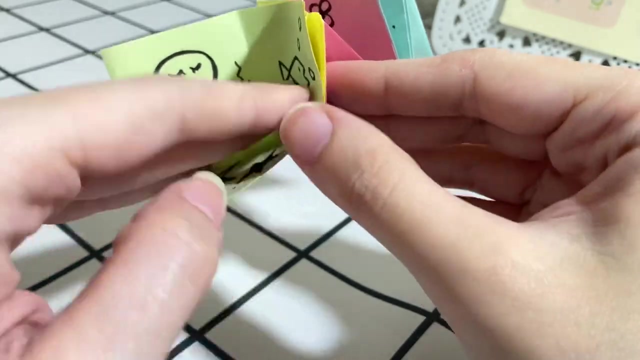 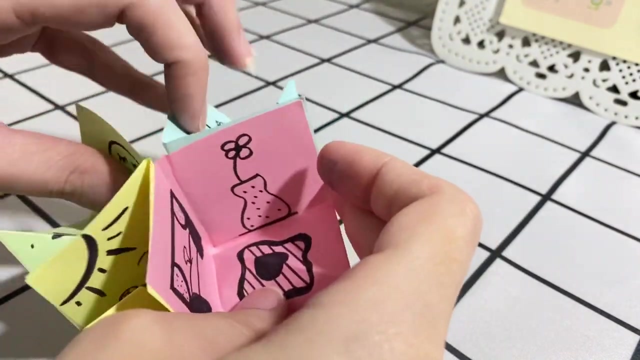 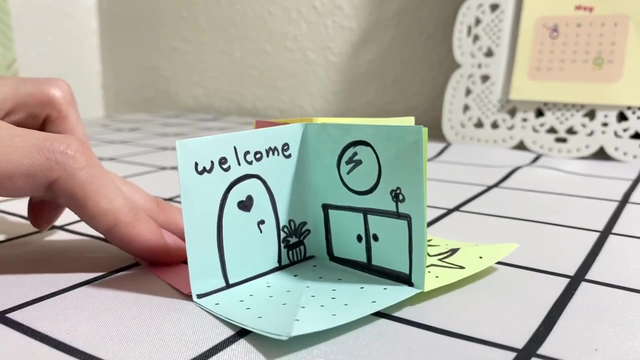 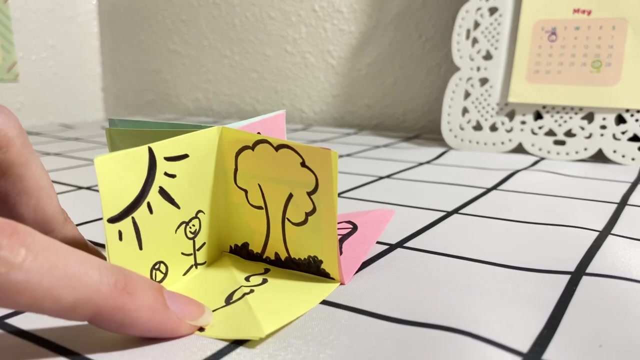 And finally, let them put their cute little fingers to let the puppet's mouth move for the sake of the video, but use regular size papers with your kids, Thank you. Thank you, Or for when you're teaching the four seasons, since it's already divided into four sections. 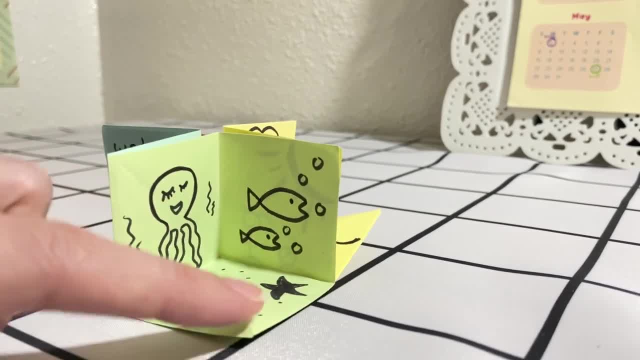 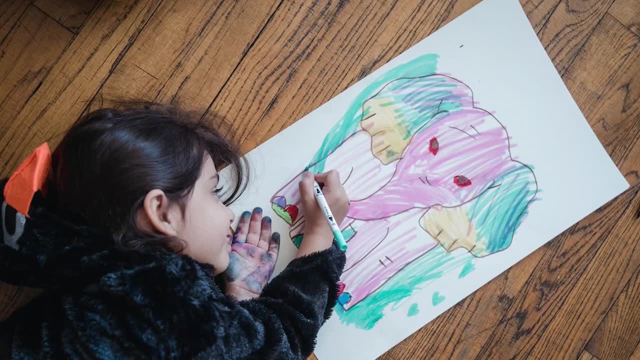 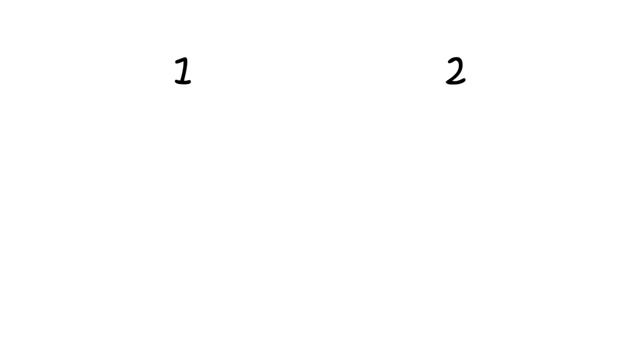 It would be great for animals and species as well. It's a simple and a great way to help internalize any new vocab words. Our last craft is called I don't know. let's go with stick and color. What I do here is I give students two sheets. 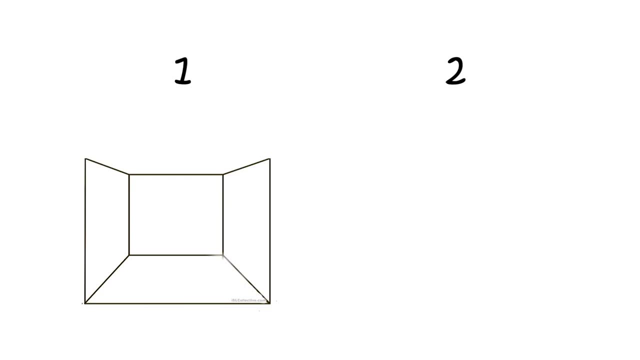 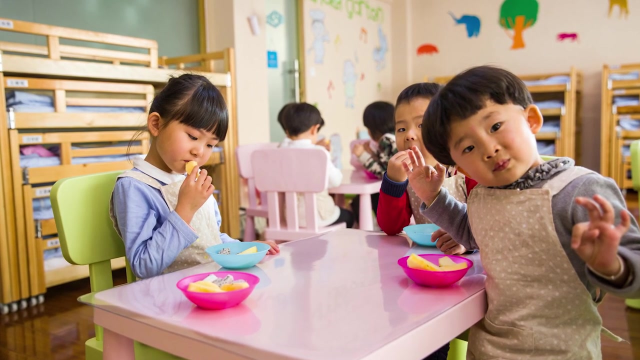 One sheet with, for example, an empty bedroom and the other sheet with bedroom objects. All they gotta do is color and then cut these objects and stick them on the first sheet to create and design their own rooms. With another group we had a lesson about food, so I used this empty fridge as my first sheet. 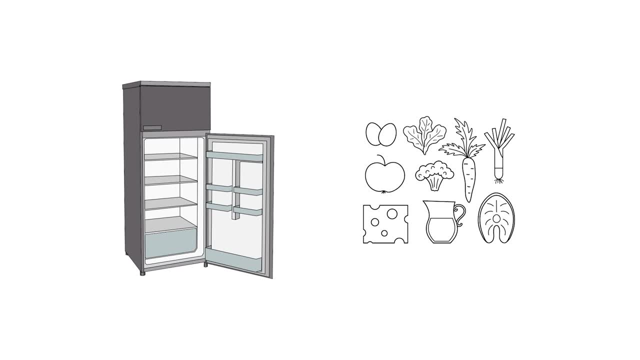 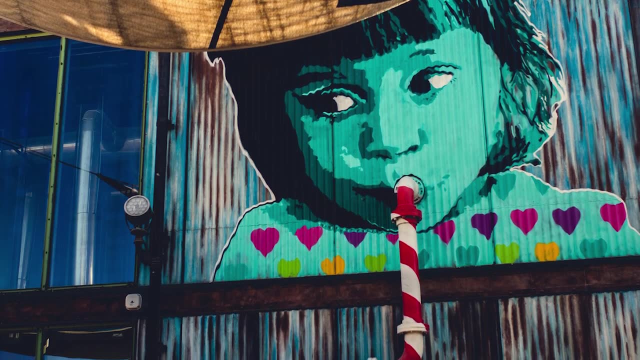 And for the second sheet we had different vegetables, fruits, snacks and beverages. I mean you can absolutely get creative here to choose whatever suits your lesson. That's pretty, it Always extra. thank you, teachers For teaching kids.